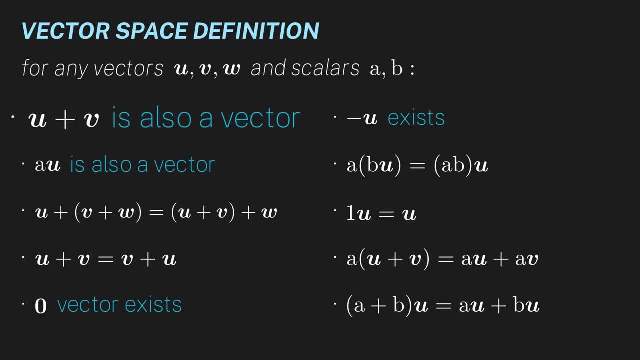 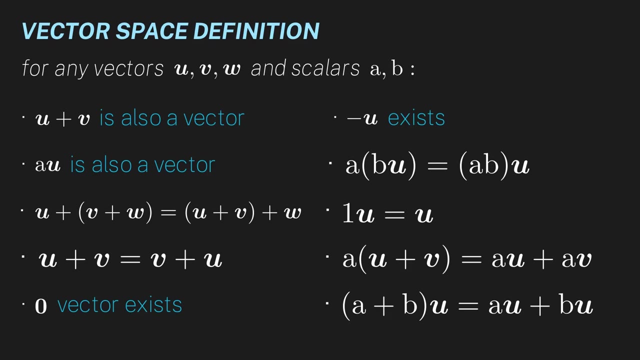 find intuitive. For example, this first one says that adding two vectors gives us another vector. The next one states that multiplying a vector by a scalar also gives us another vector, And a lot of the other ones just enforce intuitive notions about how vectors are added together. 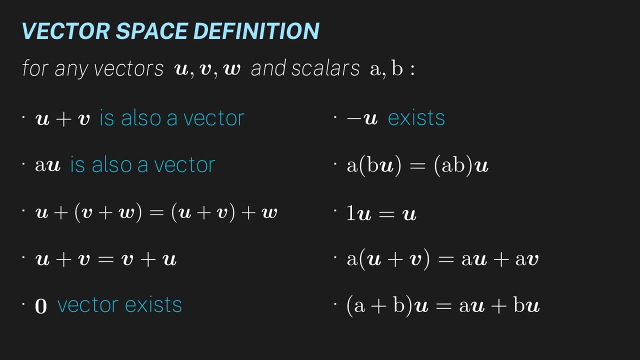 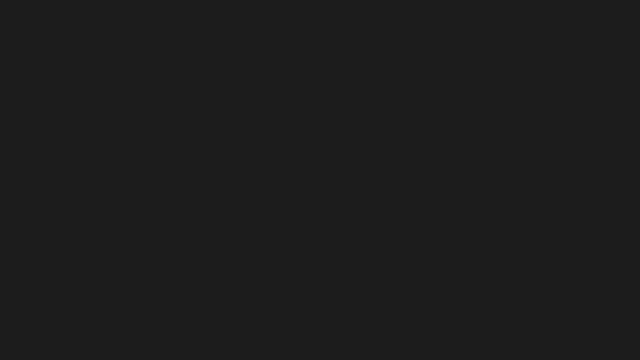 and multiplied by scalars. See how these rules just enforce what we already expect from vectors. So what is the benefit of defining a vector space like this? Well, this definition makes no mention of lists, of numbers or arrows. Any set of objects. 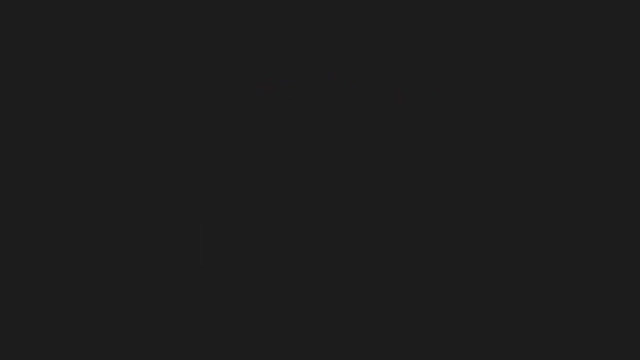 that satisfy these rules forms a vector space. With the right rules, it could be fruits, it could be functions or our familiar columns and arrows. Hopefully you're beginning to understand that linear algebra and vector spaces are all about structure and patterns, not about the type of object you're using. And it just so happens. 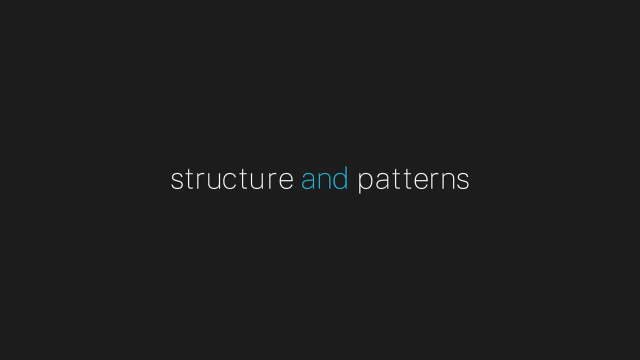 that the particular structure of a vector space is exactly what we need to describe the quantum world. So now that we understand what a vector space is, let's apply it to quantum mechanics. Like we mentioned last episode, we want our particle to be represented by a vector in 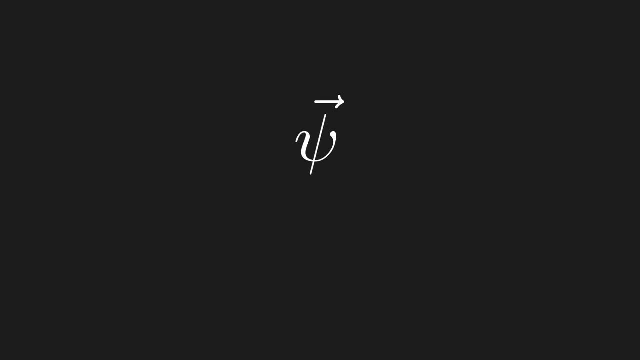 a vector space. More specifically, a vector in this vector space represents a quantum state. A quantum state is a mathematical object that holds all the physical properties of our particle. From it we should be able to extract the possible positions, momenta, energies, etc. at any. 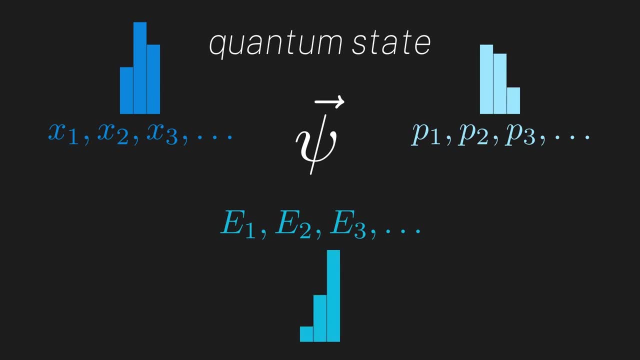 particular moment in time, As well as all the associated probabilities. Now, instead of using our typical vector symbol here, physicists like to use a different symbol for vectors in quantum mechanics, We will represent a vector using this notation here. When we write a vector in this way, we will call it a ket. 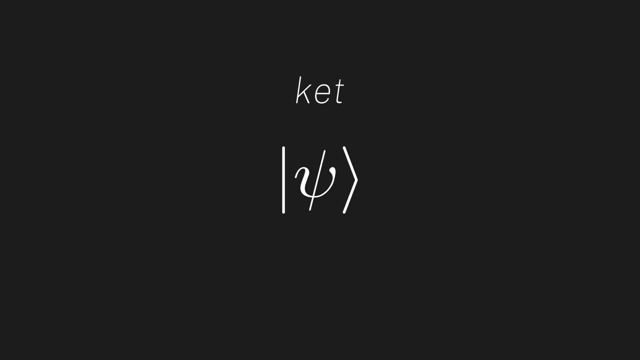 This is still a vector, it's just a different notation. The reason for choosing this notation might seem strange, but its power will become apparent in later episodes. Now let's relate this notation to quantum mechanics. Remember from last episode. we wanted to represent our particle as a linear combination of all. 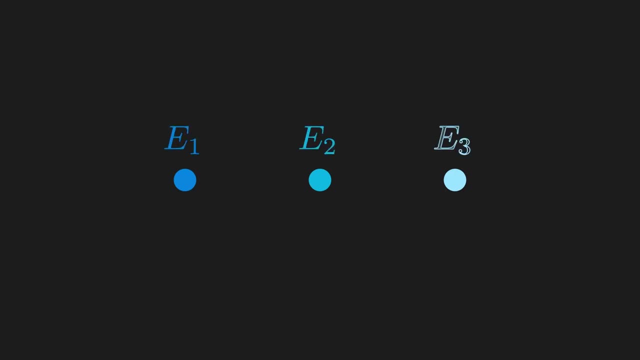 possible outcomes of a measurement, for example energy. Therefore, we would have a list of quantum state kets representing each possible energy outcome, and our present quantum state is represented by a linear combination, often called a superposition, of all these quantum states, where the coefficient has something. 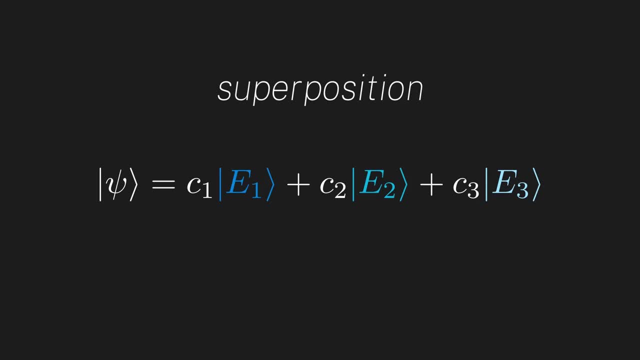 to do with the probability of that outcome. If, instead, we wanted to measure angular momentum, we would have a list of quantum state kets representing each possible angular momentum outcome and we would have a different linear combination, but still the same present quantum state, and so on and so forth. for 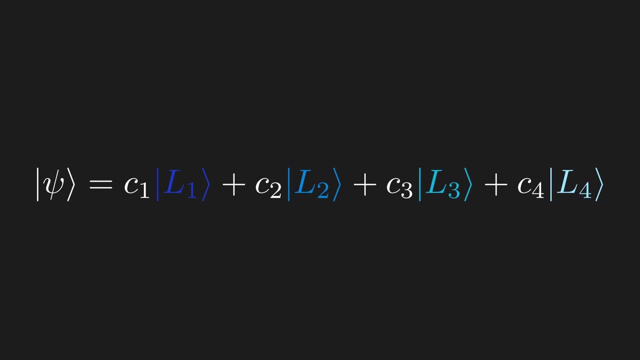 each measurement we could make. In a later episode, we'll discuss how we get these lists of outcome states and associated probabilities. Now, here we have a finite list of outcome states, but it may very well be that we have infinitely many outcomes. 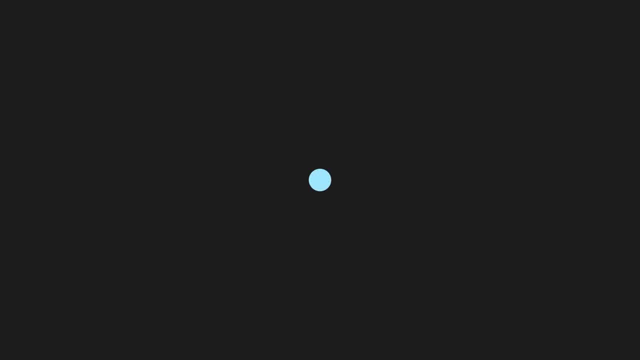 I mean, think about it. What's stopping you from giving a particle more and more energy? We need to have outcome states for arbitrarily high energies. Therefore, we may sometimes have linear combinations of infinitely many kets, representing a superposition of infinitely many outcomes. 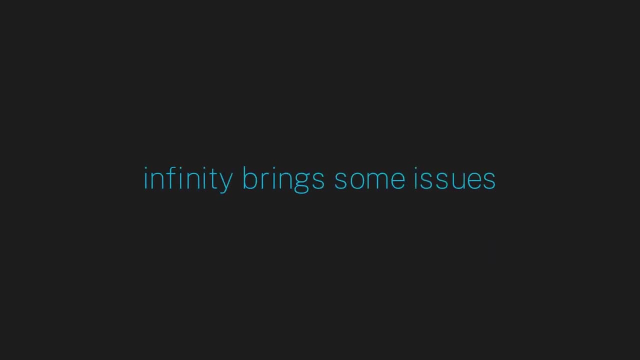 In the next episode we'll quickly discuss how this infinity brings some issues with it and why a Hilbert space fixes it. But for now, thanks for watching. Now, let's assume an infinite linear combination doesn't cause any problems, But we do have a separate issue to address. 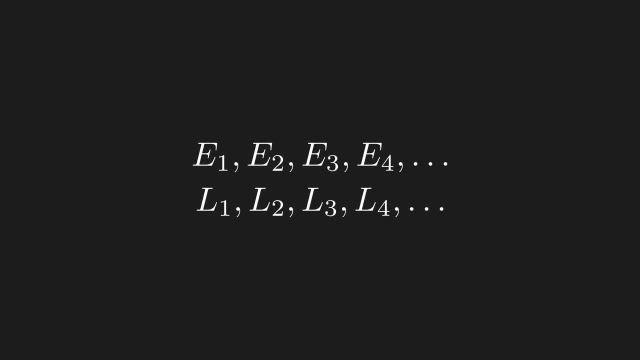 So far we've been looking at the case when things like energy and angular momentum have a discrete set of possible values. But physical quantities are not always discrete. For example, let's look at position. So far we do not have experimental evidence showing that position is discrete. 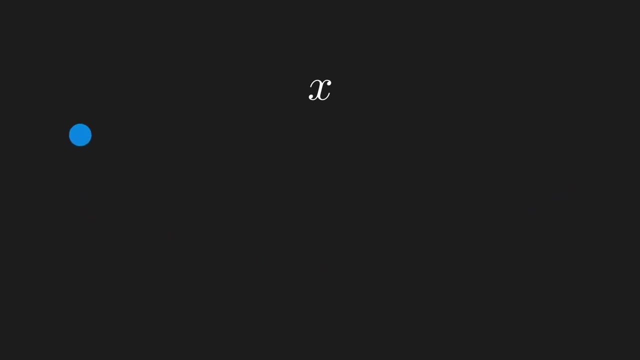 An electron can be anywhere it pleases. So far we've been looking at the case when things like energy and angular momentum have a discrete set of possible values, But we do not have experimental evidence showing that position is discrete So far. let's look at the case when things like energy and angular momentum have a discrete 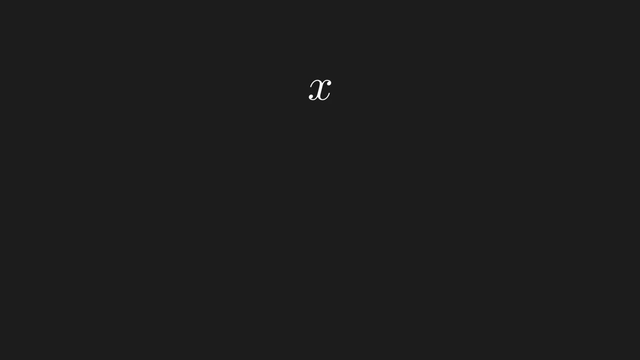 set of possible values. In other words, position is continuous, not discrete. In other words, position is continuous, not discrete. We want to be able to mathematically describe this within our theory. So here's a puzzle. Say our electron can have any possible position, although some may be more likely than others. 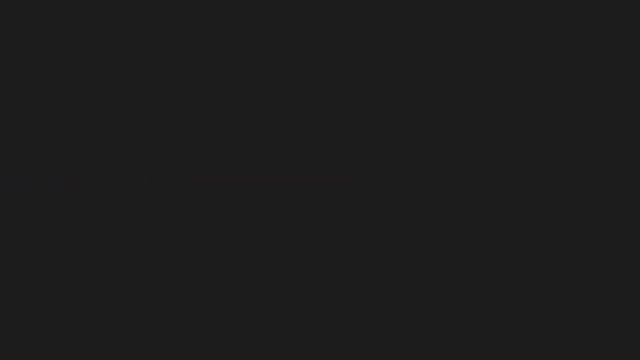 How do we represent the quantum state of our electron using the kets of possible positions? Our typical sum won't cut it, since to have a sum we need a discrete list of things to add together and it's impossible to cover all positions using a discrete list. even 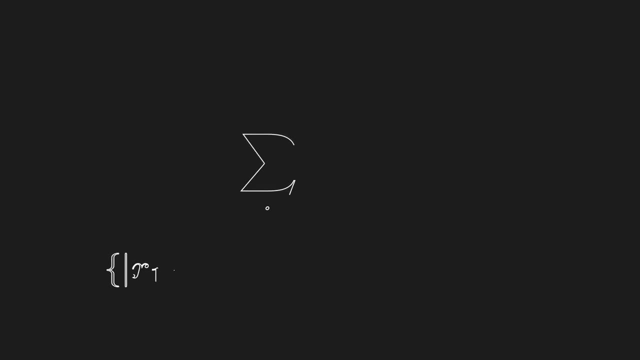 if that list is infinite. So what we need is some mathematical operation that has the power to sum over a continuous set. See if you can think of one. You might have realized that the integral is an operation that does exactly this. I mean think about it. 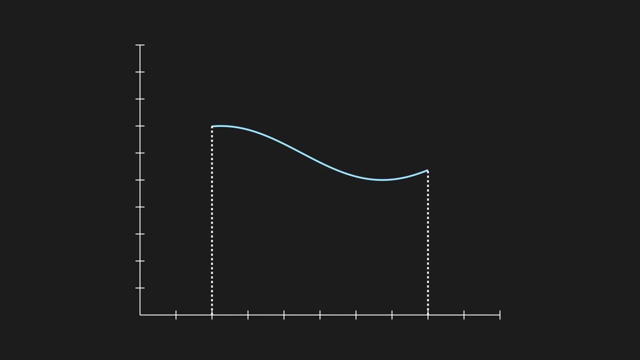 To find the area under a function. the integral adds together the contribution from each tiny slice at every point along the continuous set of function values. The integral is exactly the continuous sum we need. So let's use the power of the integral to write a linear combination when we have a. 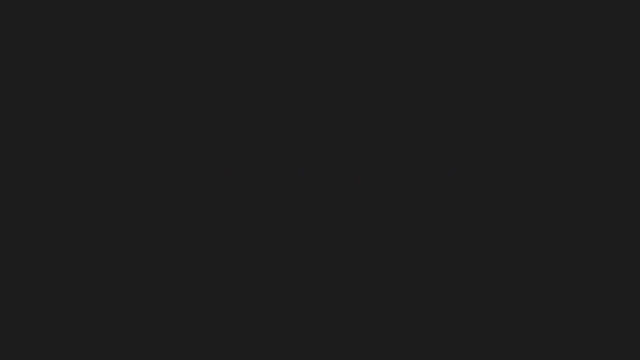 continuous set of outcome possibilities. First we want to write this as a sum, so we write the integral symbol indicating a sum. Note that the limits of integration are implicitly plus and minus infinity. Next, we are summing over all possible position outcomes represented by variable x. so we 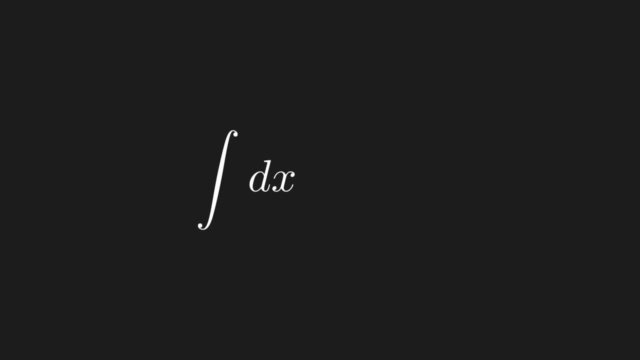 need to have a differential dx to indicate that. Don't worry about where we put the dx In many theoretical physics texts. you'll see it in front. Next we need our kets, which we will label by the position they represent: x. 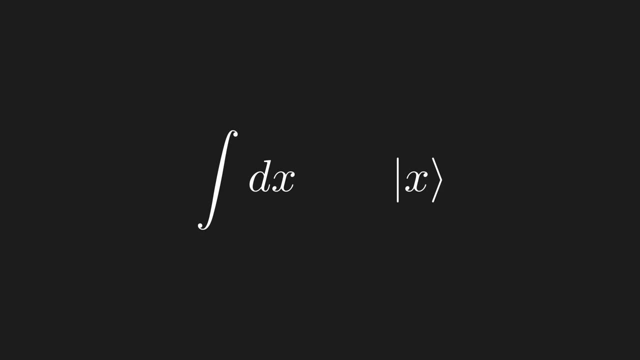 Lastly, we need our coefficients. We have a coefficient of x. We have a coefficient for every possible position, x meaning we need a number for each value of x. This is exactly what a function does, so let's use a function for our coefficients. 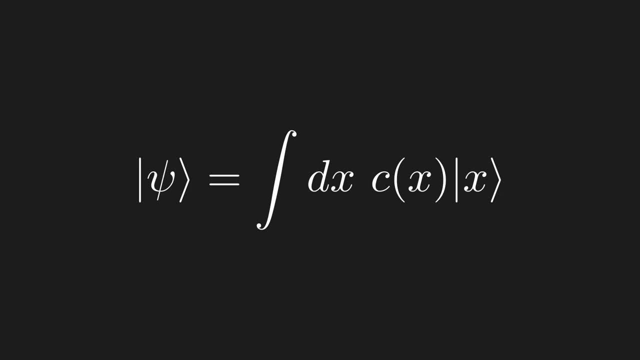 And there it is. We have written a quantum state where the superposition is over a continuous set of outcomes. This can be very confusing if you're seeing it for the first time. Just remember that an integral represents a continuous sum, so this is just a continuous. 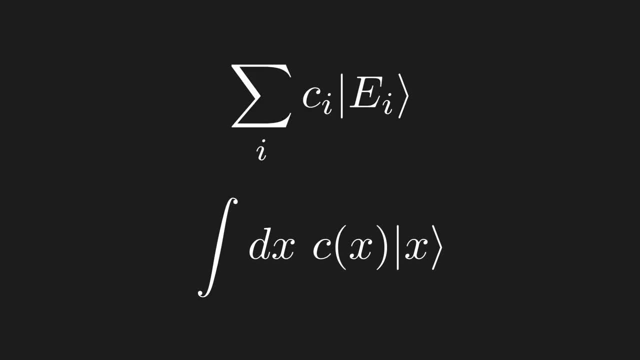 linear combination of outcomes. Comparing this to our typical linear combination, hopefully you see that one is just a continuous version of the other. Before moving on, I want to spend a second discussing the coefficient function that we have here. It may seem weird to use a function in place of a coefficient, so let's see how it comes. 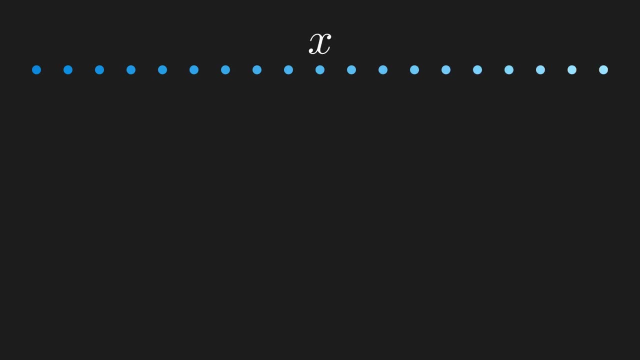 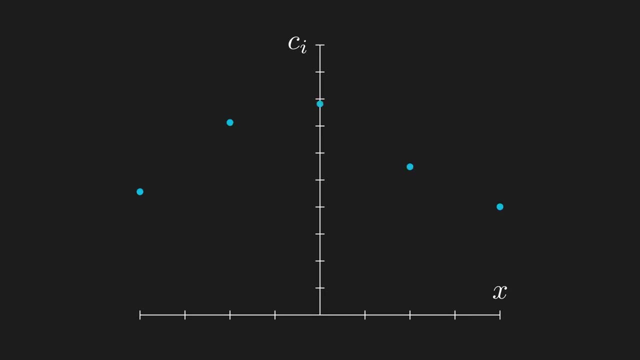 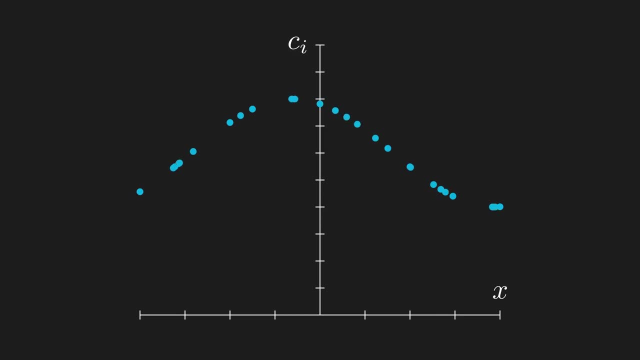 Now let's begin undiscretizing position. Let's close the gap between the possible positions, adding coefficients for all the positions that we're missing. As this occurs, the coefficients start getting closer and closer and you see that they begin forming a line. 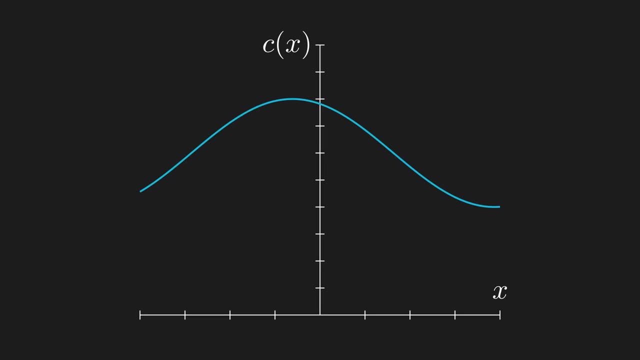 For now we just assumed this function must be continuous, but we'll justify this assumption in a later episode. See how we get the transition from discrete coefficients to function. Now let's note something important. Remember that in the linear combination of possible outcomes, the coefficients are somehow 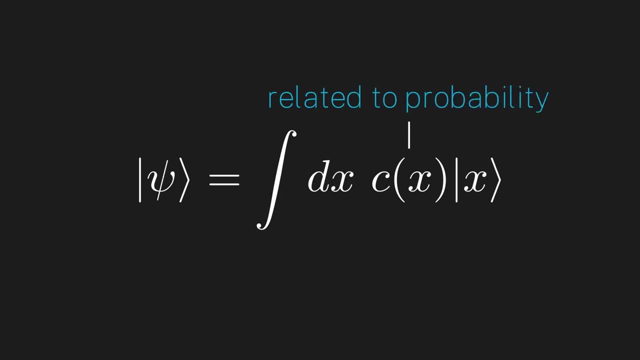 related to the probability of getting that particular outcome. Meaning this function here somehow tells us about the probability of a particular position. If you have some previous quantum knowledge, maybe you know of another function that is related to the probability of position. Your mind might have jumped to the position wavefunction and in fact this function here. 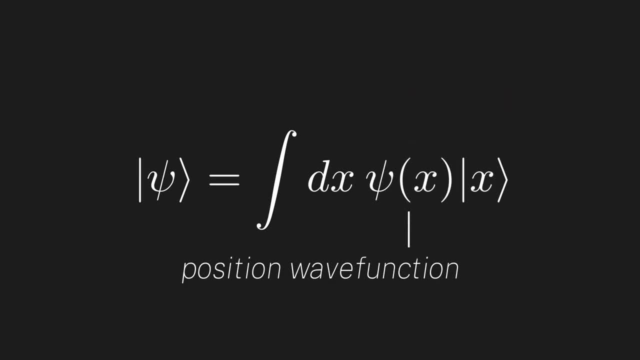 literally is the wavefunction. We'll prove this in a later episode, but take my word for it. So hopefully you see that in the linear algebra framework the position wavefunction is just the list of coefficients in the equation. When I was first learning quantum mechanics, I always wondered how functions connected 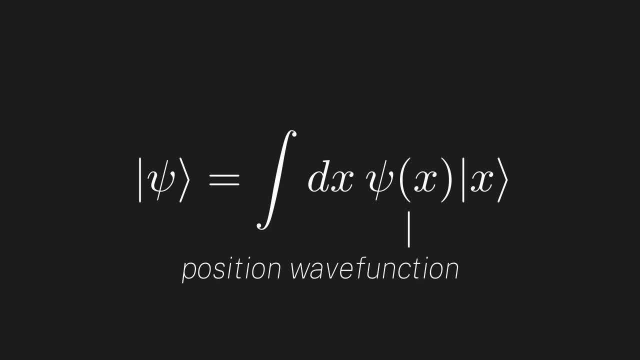 with the linear algebra framework And hopefully now you see how Many people often state that the wavefunction is a vector, Although functions can live within their own vector space and you can frame quantum mechanics in that way. now you know what wavefunctions actually represent. 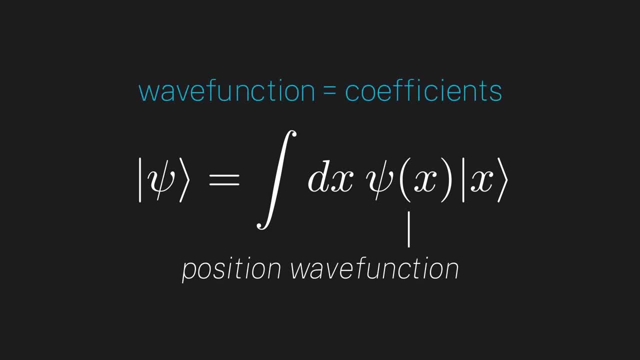 Wavefunctions in quantum mechanics represent coefficients to kets whenever the list of kets is continuous. Now, what do these coefficients have to do with waves? For that you have to wait until we derive the Schrodinger equation. So be patient.